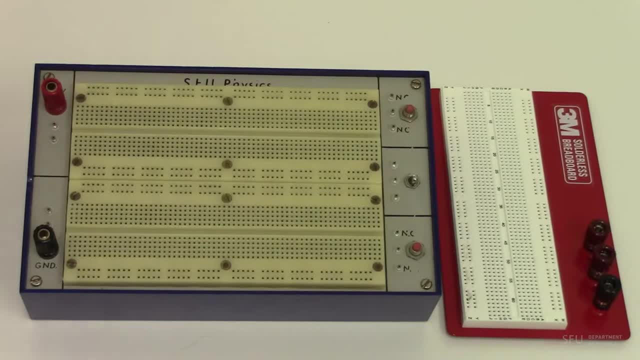 them useful to build your diode circuits In the lab. you will see the two breadboard styles here. Though they are slightly different, the underlying layout pattern is the same. Let's look more closely at the blue breadboard. It is composed of bus strips and terminal strips. 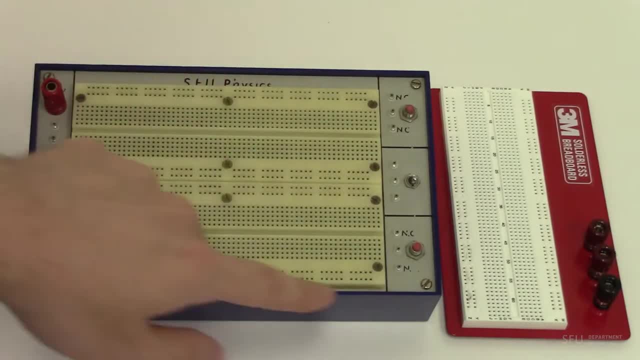 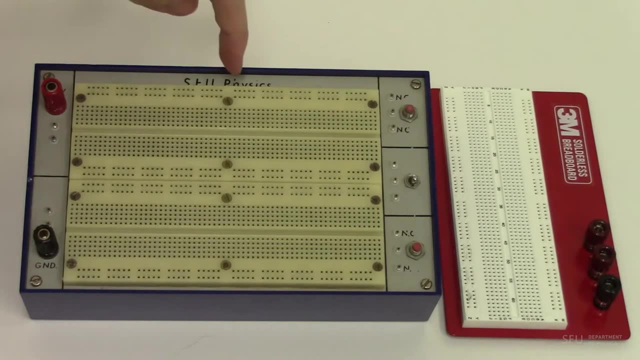 The bus strips here, here and here are all connected horizontally but not vertically. The gap in the middle here indicates that the bus strips on the left are not connected to the bus strips on the right, The terminal strips, on the other hand. 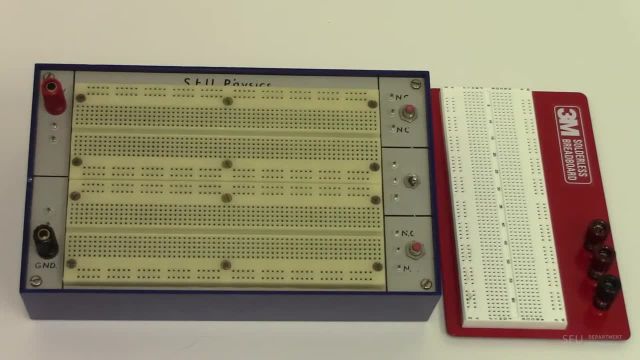 here and here are connected vertically but not horizontally. Again, the gap in the middle indicates that the top terminal strips here and the bottom terminal strips here are not connected. It's common to run power and ground connections through the bus strips and put electrical 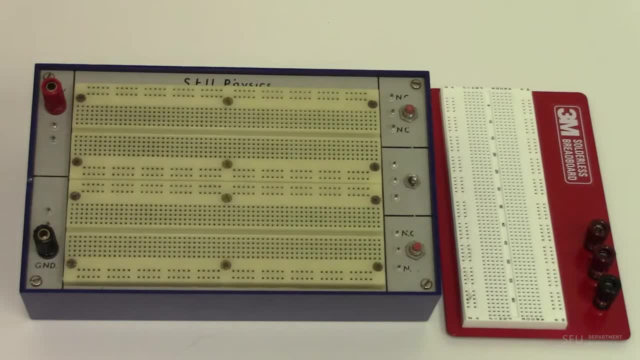 components in the terminal strips. To make a connection, you just poke a wire in like, so You only need to put in maybe half a centimeter or at most a centimeter of wire. Occasionally you might find that the hole in the breadboard is a little too tight for the wire. 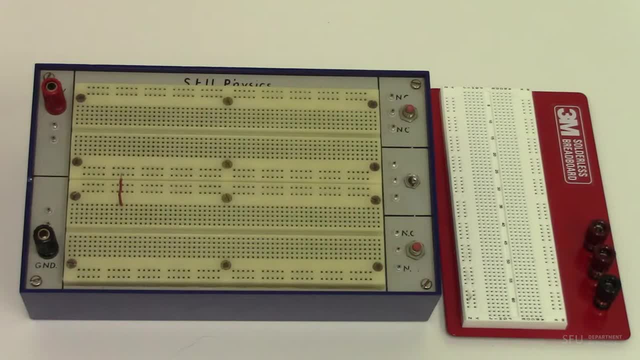 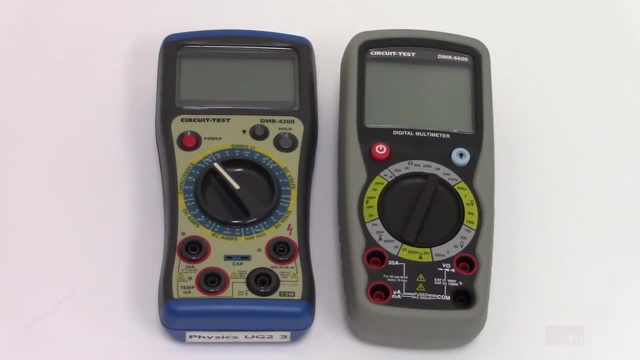 in which case you might want to use a pair of pliers to push the wire in. These are our hand-held digital multimeters, or DMMs for short. We have two models in the classroom: one blue and one gray. They operate the same way, though they have slightly different technical specifications. 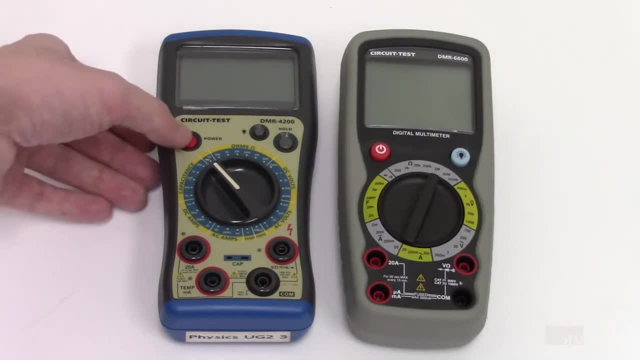 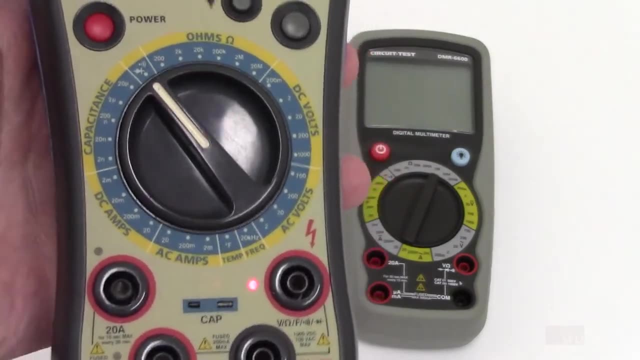 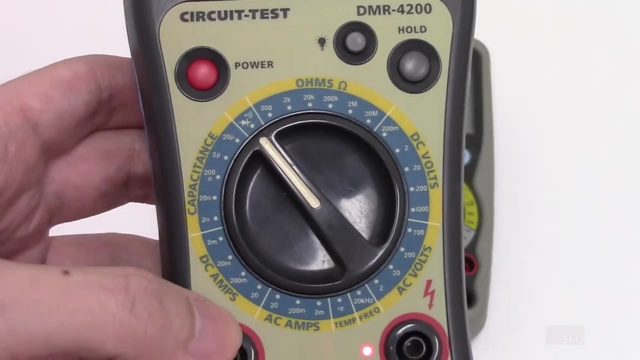 Let's take a closer look at the blue. one Power switch is here and in the middle the dial for selecting the measurement mode. Of most interest to you in this lab are probably the resistance measurements, DC voltage measurements, direct current measurements. and finally, the diode test On the bottom. here are the terminals where you take your measurements. They all accept the data connector Which is shown here. You want to use these two terminals for voltage resistance and diode measurements. Once you use these two terminals for small current measurements smaller than 200 milliamps- 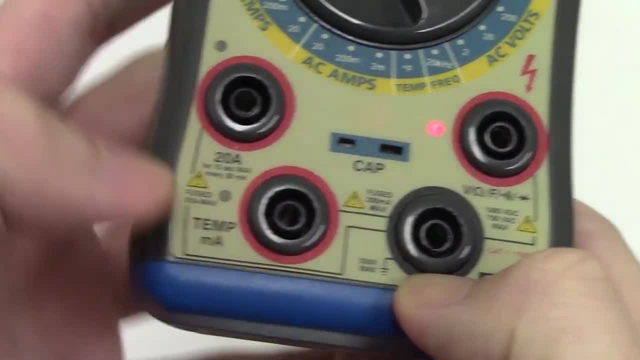 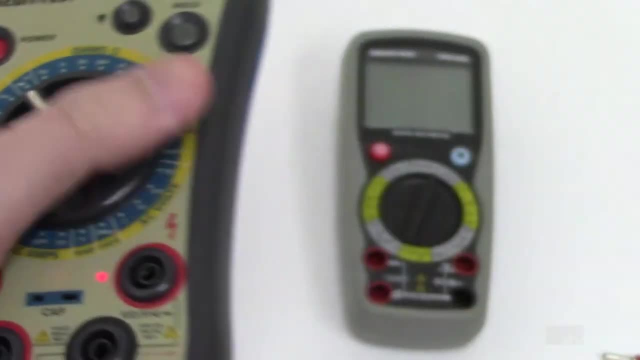 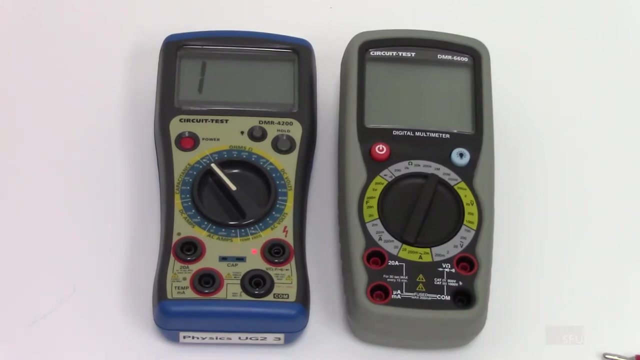 and you want to use these two terminals for large current measurements, larger than 200 milliamps. Now, both of these DMS do have fuses and if you improperly used the low current measurement terminals, you will blow that fuse If you find that your low. 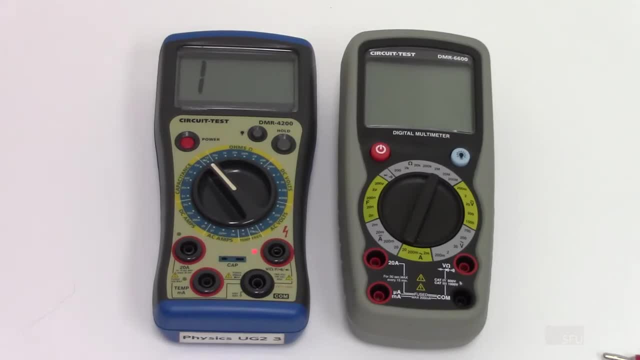 current measurement terminals do not work, then talk to your instructor or the technician to check whether the fuse has been blown. If you have blown a fuse, please check your circuit before using the DMM again. One additional note in one repetition of the experiment. 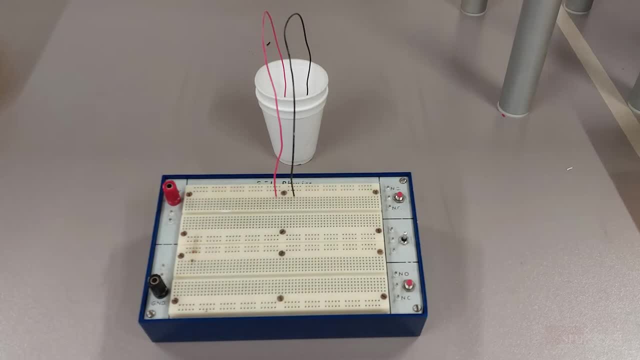 you will be cooling the diode with liquid nitrogen, so we need to go over its safe handling. The diode has long wires attached to it so that you can do measurements and position the diode while it is in liquid nitrogen If you need to move the liquid nitrogen more than a little bit. 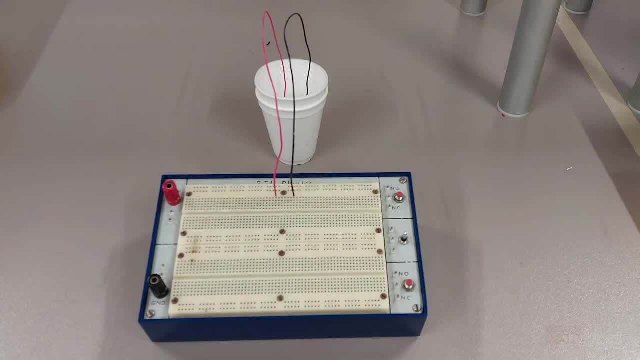 please borrow safety gloves and glasses to do so. Liquid nitrogen is both a supplication hazard and a cold hazard. Skin contact with liquid nitrogen or cold objects can cause frostbite. Except for the cold, it can also cause frostbite. If you have a cold, it can cause frostbite. 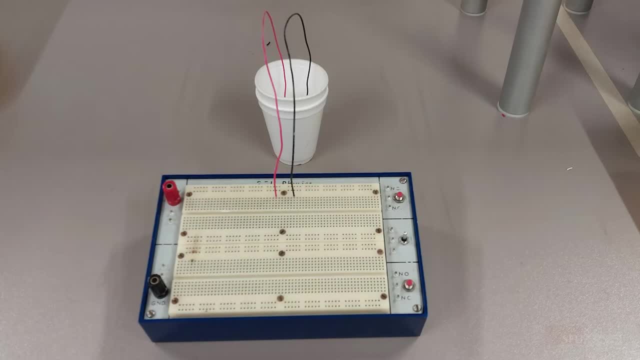 If you have a cold, it can cause frostbite. Except for the cold, it can cause frostbite. Extreme cold can make objects unexpectedly hard and brittle, so handle cold objects with care. SFU personnel will give you a styrofoam cup of liquid nitrogen and refill it as needed. 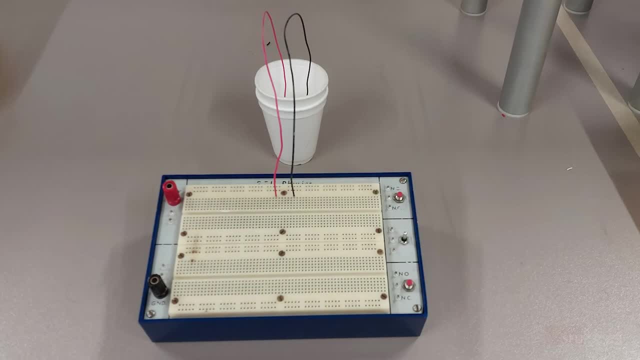 Please keep the liquid nitrogen in the main lab room where there is good ventilation. While unlikely you could experience oxygen deprivation. Symptoms of low oxygen include headache, dizziness, nausea and fatigue. If you feel unwell, don't hesitate to leave the room in. 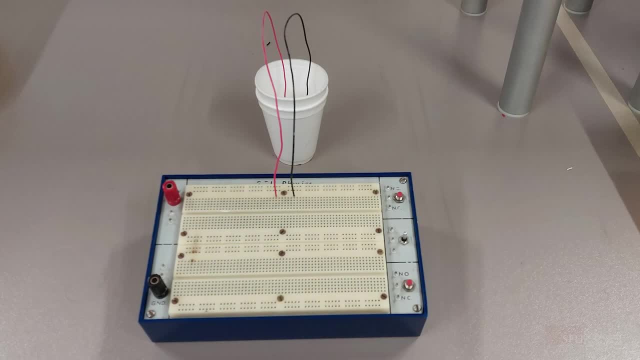 immediately warn others and report the problem. If you feel unwell, don't hesitate to leave the room in, immediately warn others and report the problem. If you feel unwell, don't hesitate to leave the room in, immediately warn others and report the problem.